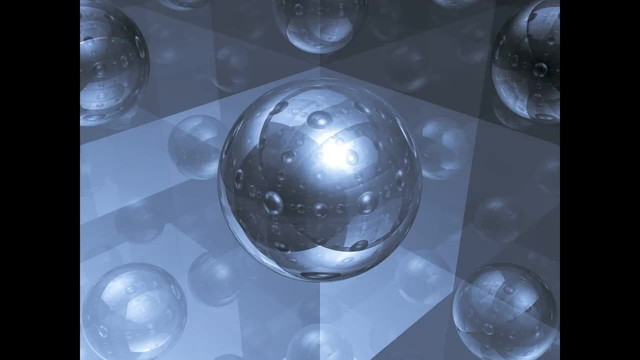 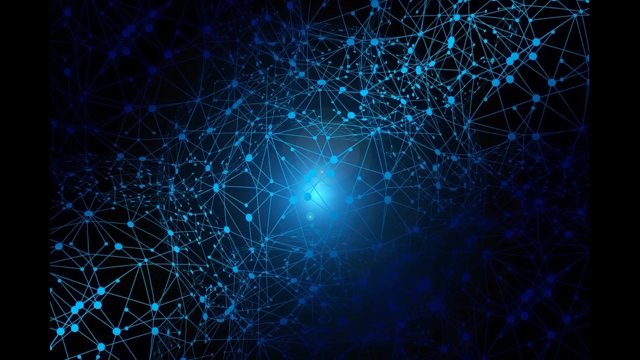 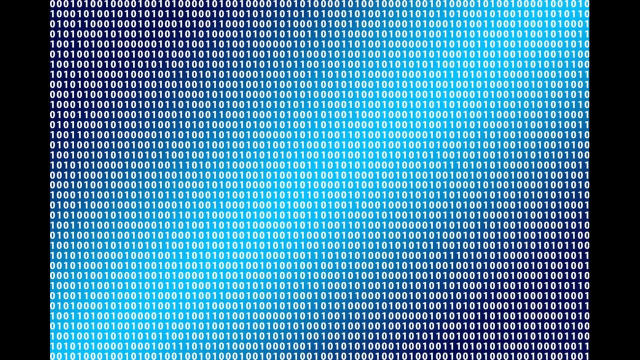 knowledge to create robust and hack-proof communication systems. The backbone of quantum cryptography is a concept that seems almost magical: quantum entanglement. According to quantum mechanics, two or more particles can be entangled, a peculiar state where the properties of one particle instantaneously influence the properties of the other, no matter the distance. 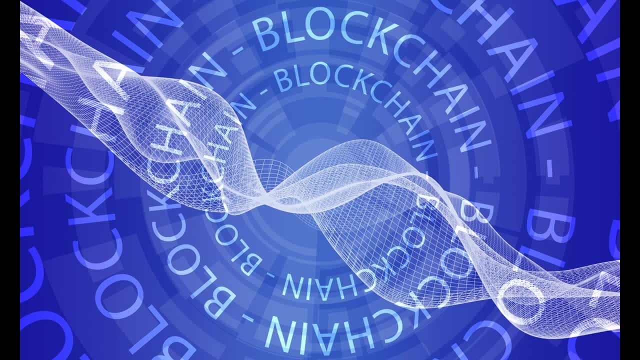 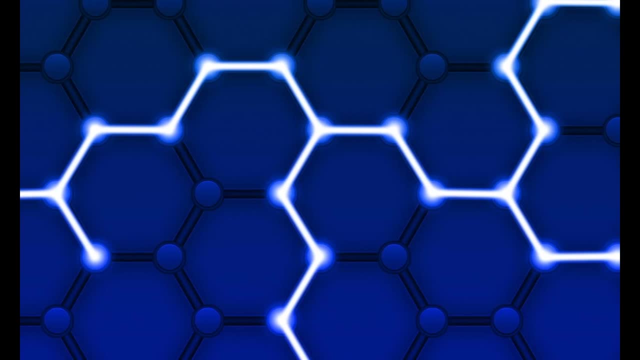 separating them. This phenomenon is what Albert Einstein once famously referred to as spooky action at a distance. The principle behind quantum cryptography is relatively simple. Consider a sender, Alice, and a receiver Bob. Alice sends quantum information to the receiver Bob and Alice sends quantum information to the receiver Bob. 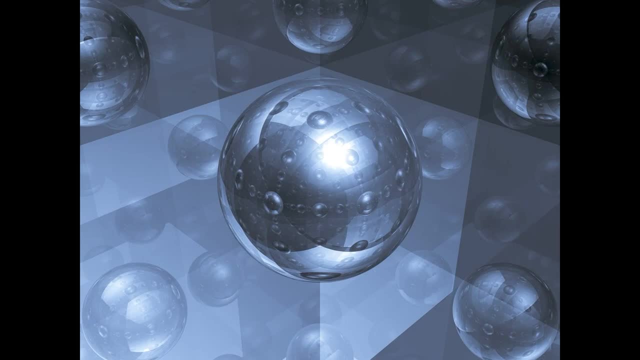 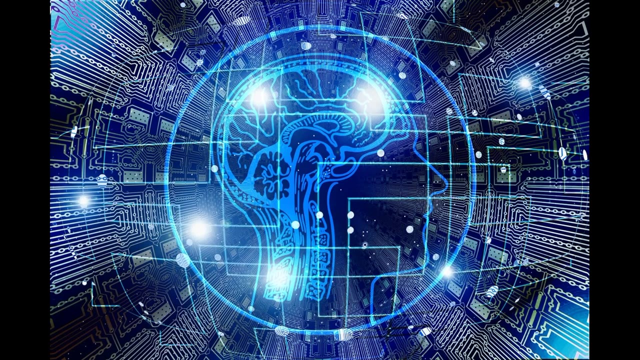 Alice sends quantum information- qubits, over a quantum channel. Each qubit, unlike classical bits, can exist in multiple states at once due to superposition, another fundamental concept in quantum mechanics, A key attribute of qubits that makes them ideal for secure communication. 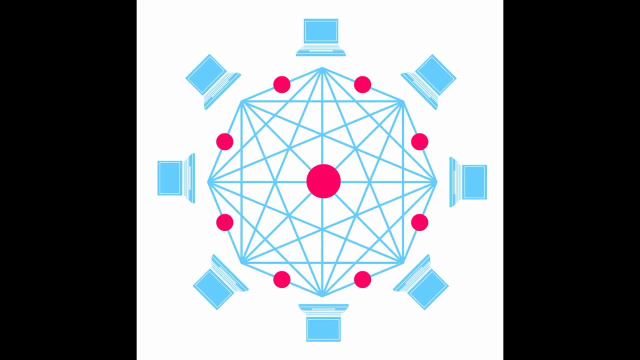 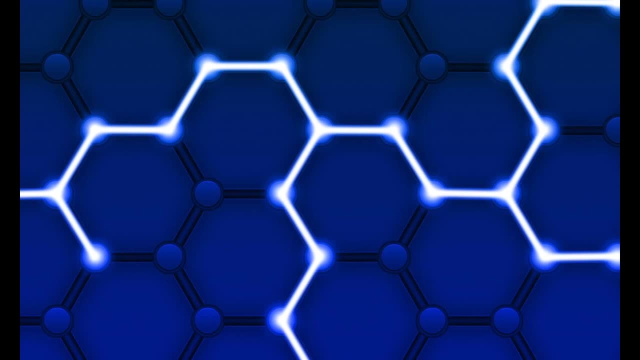 is the no-cloning theorem. It states that it's impossible to create an exact copy of an unknown quantum state. In terms of cryptography, this means that any attempt by an eavesdropper Eve to intercept the quantum communication would invariably alter the qubits. 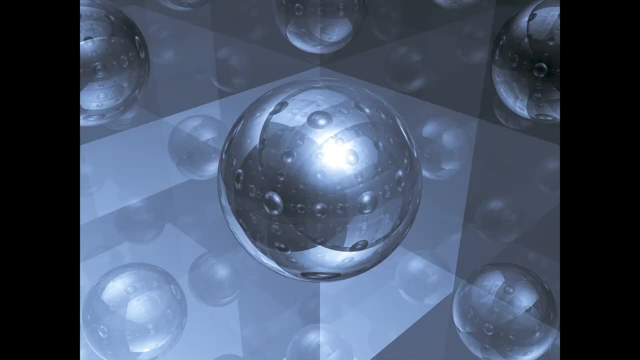 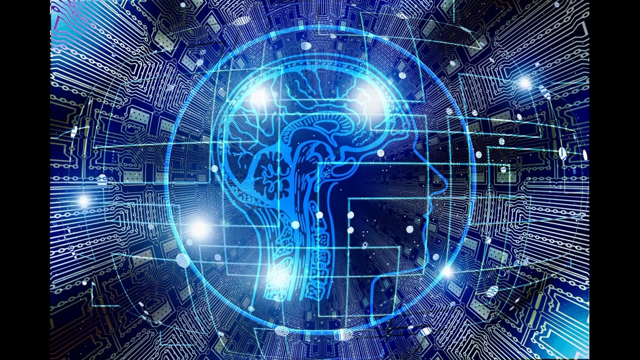 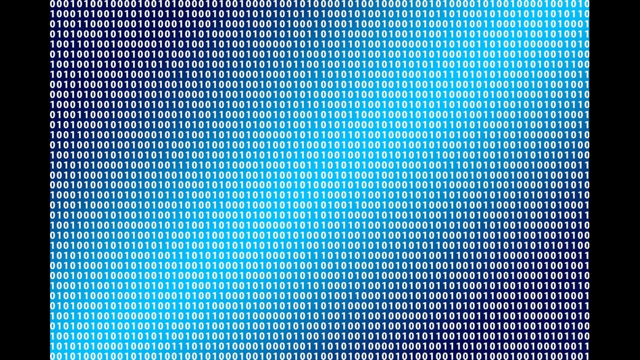 Thus revealing her presence. This leads us to a concrete application of quantum cryptography, quantum key distribution, QKD. The best known protocol of QKD is BB84, developed by Charles Bennett and Jill Brassid in 1984.. Alice and Bob use a string of qubits to 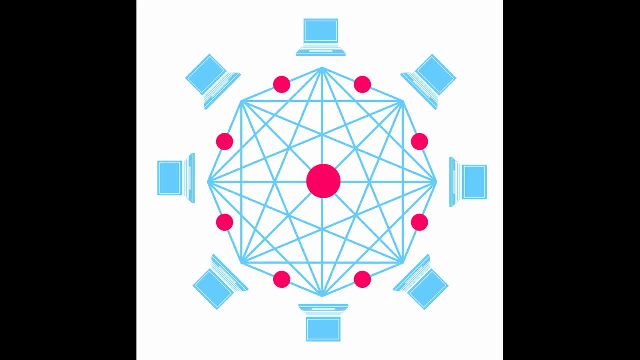 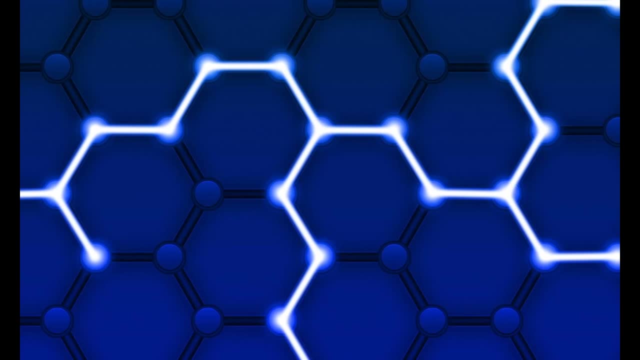 establish a shared secret key. If Eve tries to intercept her, interference will be noticed due to the change in qubit state. Thus, Alice and Bob can safely discard compromised keys, retaining only those exchanged without any interference. Quantum cryptography holds great promise for the 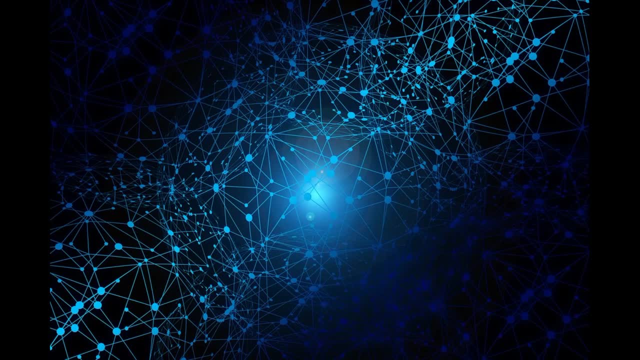 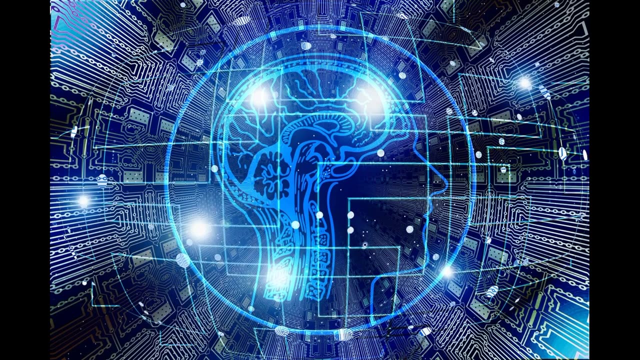 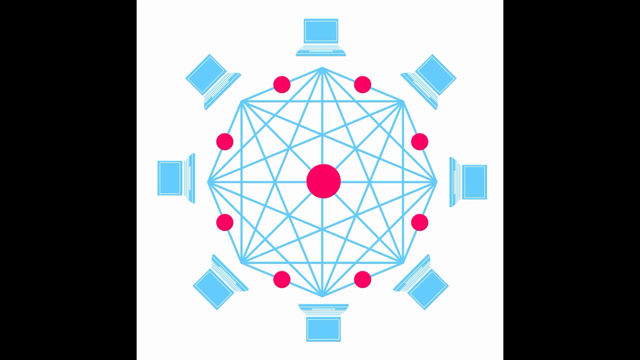 future. given the growing threats of cyber attacks. In a world becoming increasingly connected, we need ever more sophisticated methods to secure our information. However, quantum cryptography is not without its challenges. Implementation is complex and requires advanced technology, including quantum channels and detectors, Also maintaining quantum states without disruption.